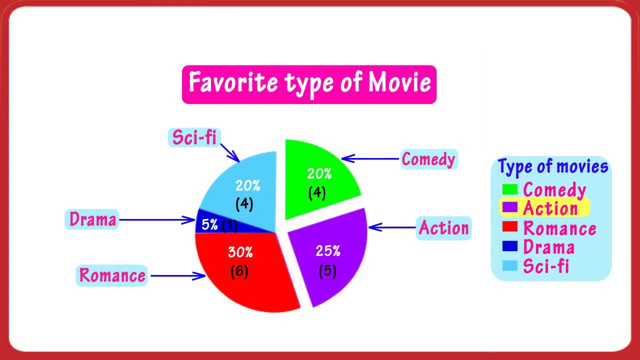 Now labels on the graph tells: purple portion represents the fraction of people that likes action movies. Label also says 5 people, which is 25% of 20 people like action movies. So percentage of circle that each portion represents says that much percentage out of the total number of people like that type of movie. 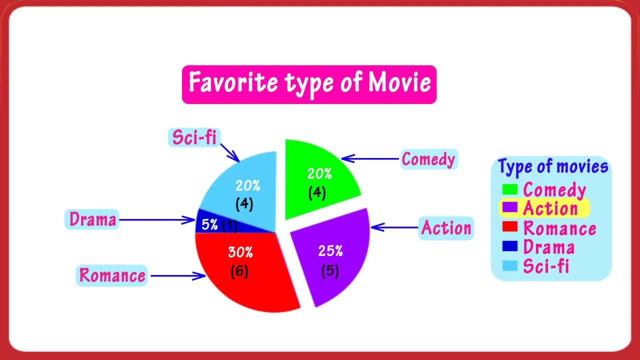 Now labels on the graph tells: blue portion represents the fraction of people that likes drama movies. Label also says 1 people, which is 5% of 20 people, likes drama movies, And so on. So when we have to show percentage values, we use a pie chart. 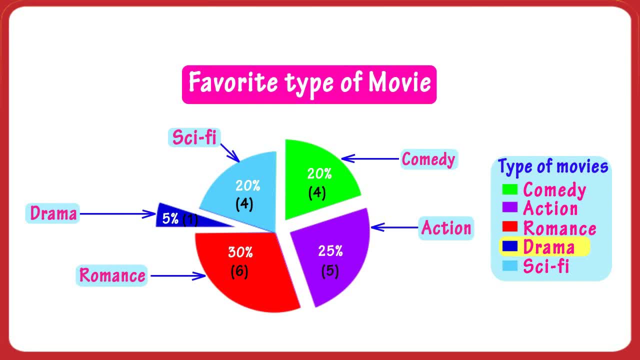 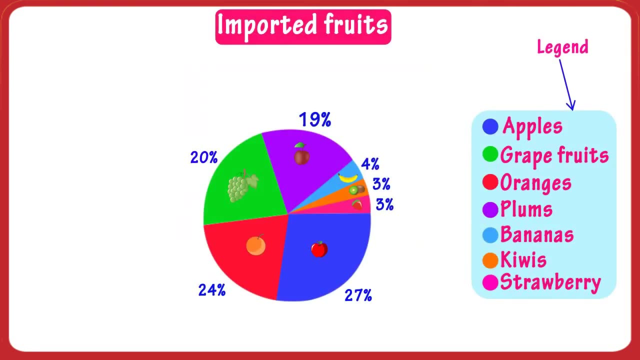 Where the percentage portion of a circle represents the percentage value And the whole set of things are represented by a whole circle. Now let's learn another example. Here we have a pie chart. Let's read it Here. the title says it is about the imported fruits. 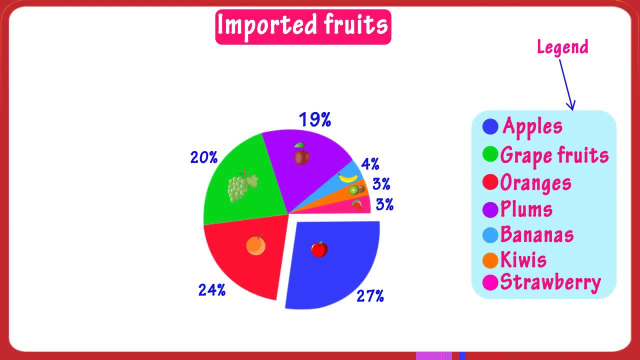 And according to labels. this portion shows percent of apples imported out of total fruits imported. The percentage of apples imported out of total fruits imported is 27%. The percentage of oranges imported out of total fruits imported is 24%. The percentage of bananas imported out of total fruits imported is only 4%. 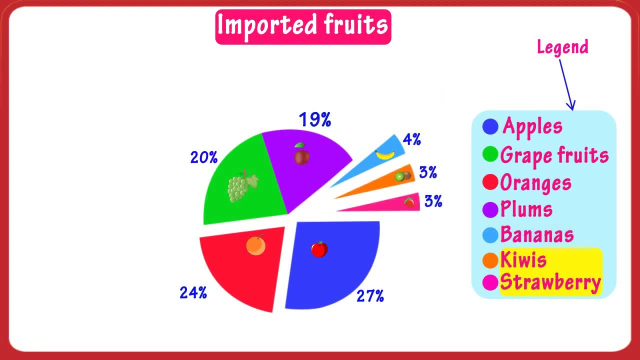 And fruits which are imported least are kiwi and strawberries, And their share out of total fruits imported is only 3% each, Which is least of all fruits, And the fruit that is imported the most is apples, which is 27%. So, kids, let's take another example. 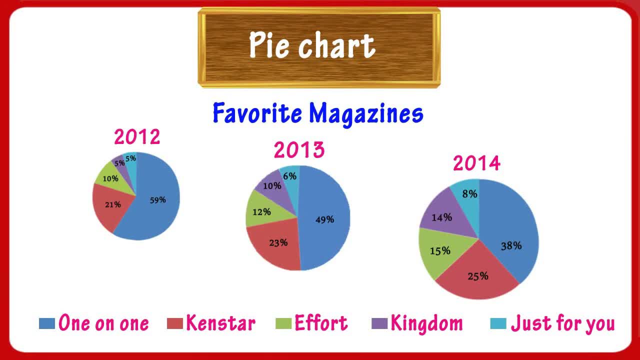 Here we have a pie chart for sale of three different years: 2012,, 2013, and 2014.. And ki shows that different colors represent different magazines sold. So each pie chart shows the percentage sale of different magazines in a year. 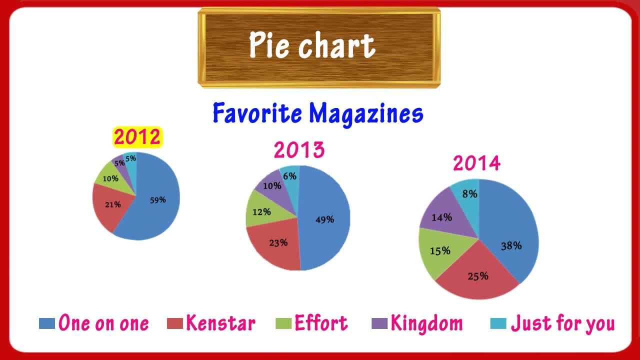 Like in 2012,, 59% of users subscribed one-on-one magazine. 21% users subscribed chemstar magazine. Now, from the three pie charts shown, we can clearly conclude that subscribers of one-on-one are decreasing: 59%, 49%, 38%. 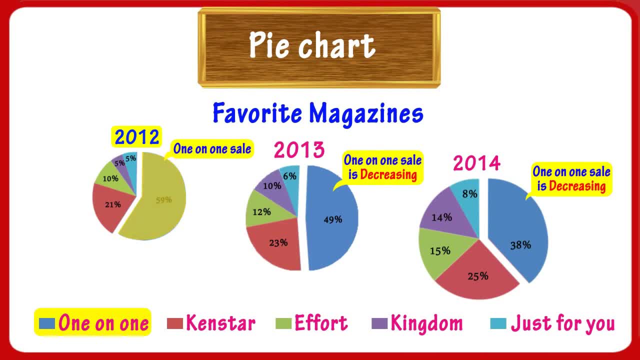 In 2012,, 59% of people subscribed to one-on-one magazine. In 2013,, 49% people subscribed one-on-one magazine. In 2014,, 38% of people subscribed one-on-one magazine, So its subscribers are decreasing. 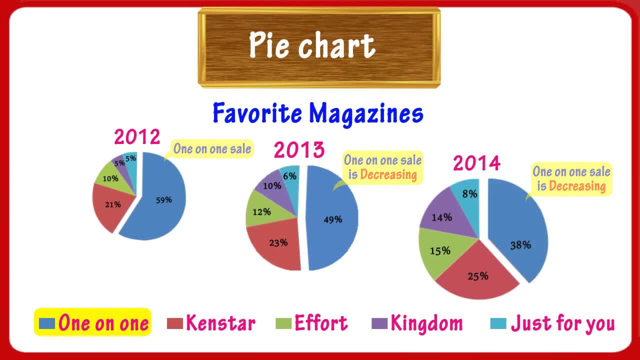 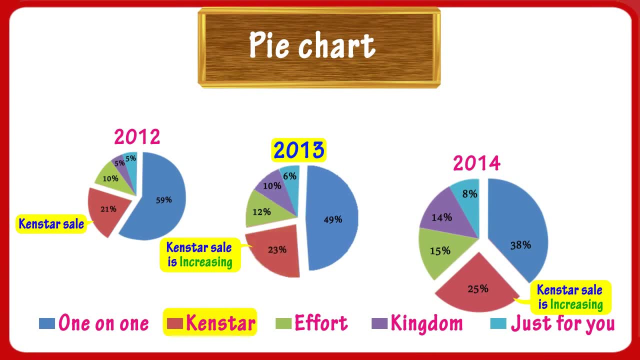 And subscribers of chemstar are increasing: 2012,, 21%, 2013,, 23%, 2014,, 25%. More trends can be easily Like. subscribers of effort are increasing 2012,, 10%, 2013,, 12%. 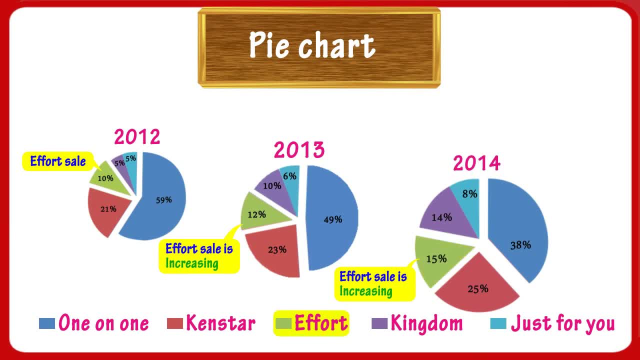 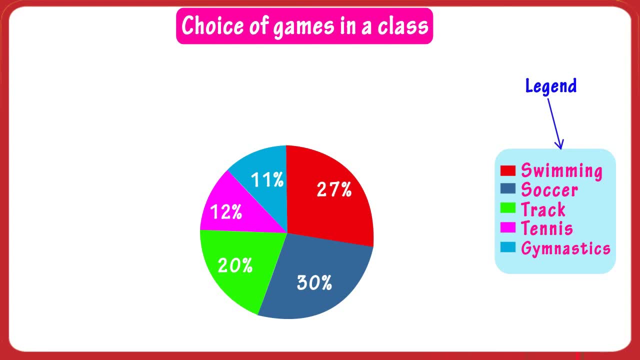 2014, 15%. Here is another example of pie chart. Here this pie chart is giving us percent of students opting for different games, Like, 11% students out of total students are opting gymnastics. 12% of students are opting tennis. 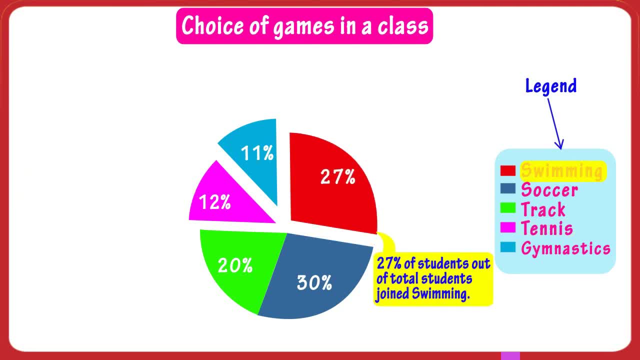 27% of students are opting for swimming. Remember pie chart always show how a whole is divided up And the whole circle always show the total number of things, Like total number of students in this example, And the slices show the percentage values.